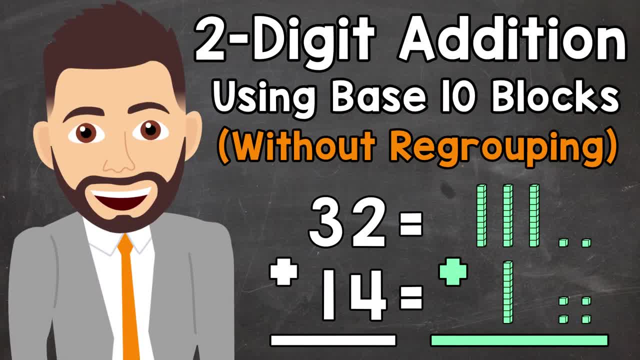 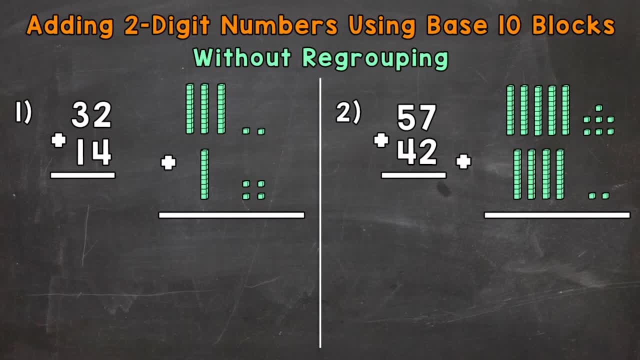 Welcome to Math with Mr J. In this video, I'm going to cover adding two-digit numbers using base 10 blocks, without regrouping, And we have two examples that we're going to go through together in order to get this down. Now, using base 10 blocks is going to help us visualize these. 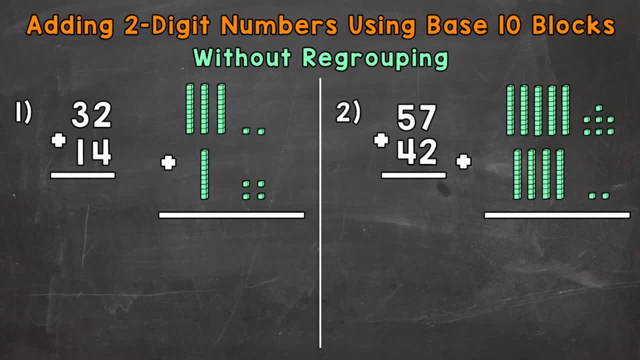 addition problems. It's also going to help our overall understanding. So let's jump into number one, where we have 32 plus 14.. Now the base 10 blocks that represent those numbers are, to the right, 32 up top and then 14 down below. Our ones are lined up and the tens are lined up. 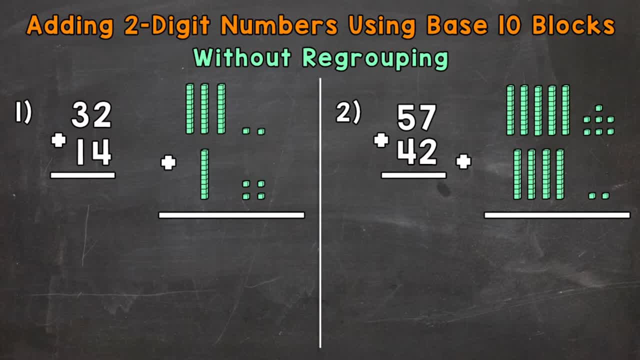 Now, when we add, we always start with the ones, So we start with 2 plus 4.. So we have two ones from 32, a 2 in the ones place, plus four ones from 14, a 4 in the ones place. So 2 plus 4 is going to give us well, 1,, 2,, 3,, 4,, 5, and 6 ones, 2 plus 4. 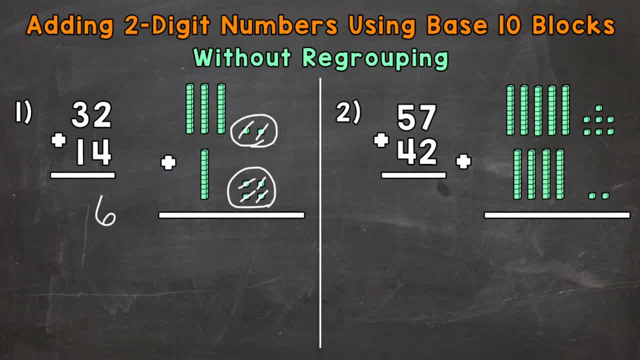 is 6.. Now for the tens, So 32, we have 3 groups of 10.. That 3 represents 3 groups of 10, or a value of 30. Now the 1 in 14 represents 1 group of 10, which has a value of 10.. 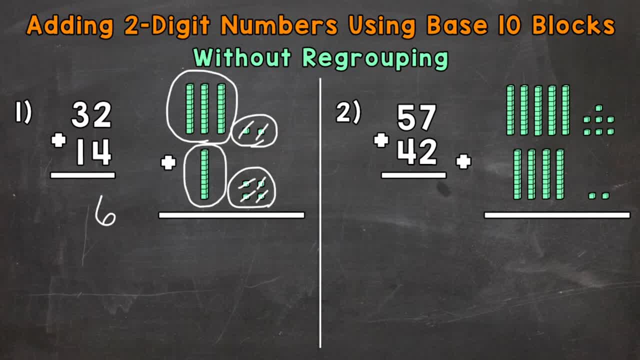 So that's represented right here. So we need 3 plus 1.. That's going to give us 1,, 2, 3, 4 groups of 10.. So we put a 4 in the tens place And our final answer is 46.. Now the 4 in 46. 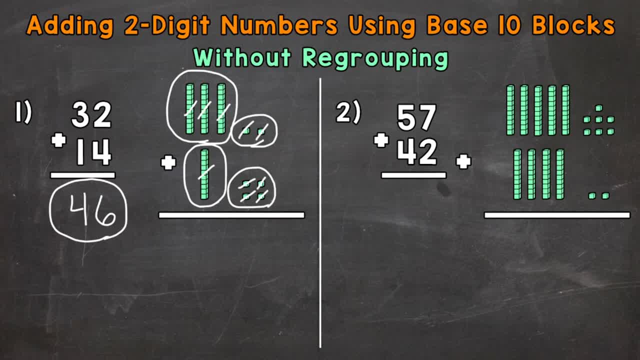 represents those 4 groups of 10. And has a value of 40. The 6 represents those 6 ones and has a value of 6.. Let's move on to number 2, where we have 57 plus 42. Again, we always start with the ones. So 57, we have a 7.